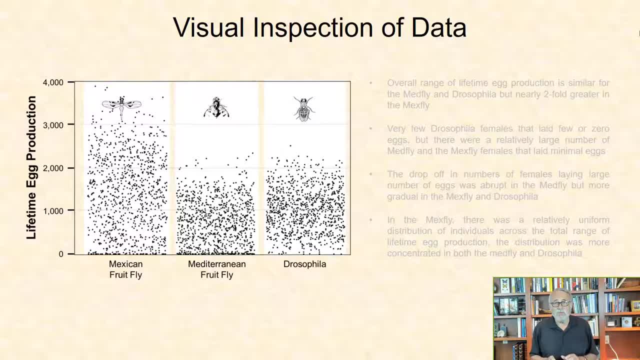 the experimental results reveal new discoveries that need to be replicated or validated. As an example, consider the scatterplots of the lifetime reproductive data for three-year-old children. These are the ones that are most likely to be collected. These are the ones that are most likely to be collected. 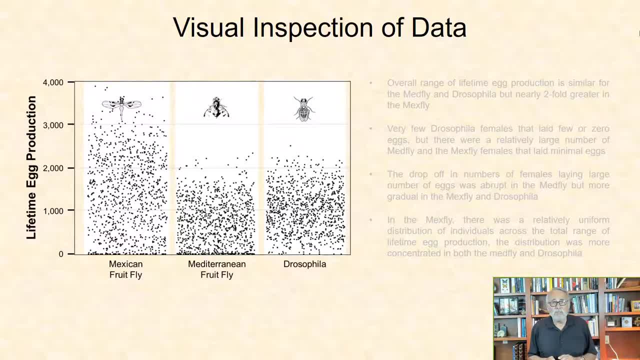 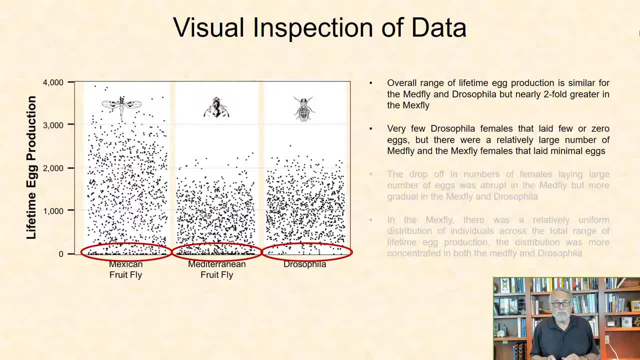 With respect to infertility, there were very few drosophila females that laid few or zero eggs, but there were a relatively large number of medflies and the Mexican fruitflies that laid either no eggs or a minimum number. With respect to high reproduction, the drop-off in numbers of females laying large numbers of 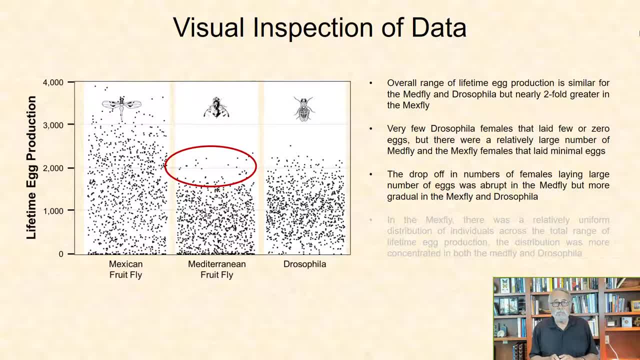 eggs was abrupt in the medfly, but more gradual in the mexfly and drosophila. The data shows that, whereas in the mexfly there was a relatively uniform distribution of individuals across the total range of lifetime egg production, the distribution was more concentrated in both the medfly and drosophila, with drop-offs at both high and low values. 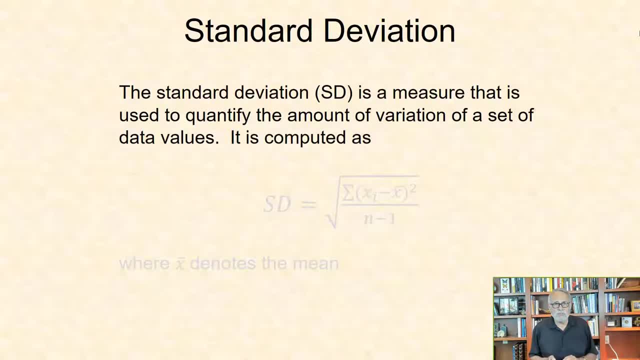 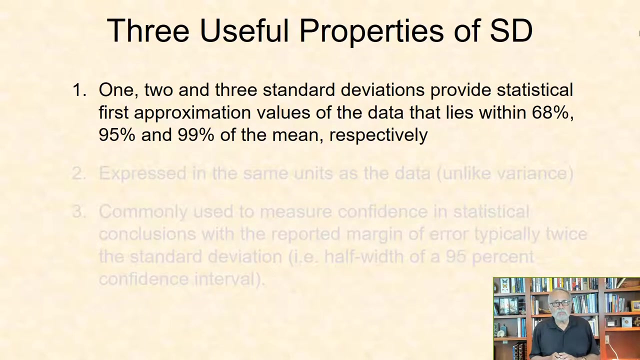 So there was significant lay over average Hiest javelin observed. for those of you in the Medboss group that answered as well. considering that the American maplers are by no means true, The way we measure quantity participation Same as one can average high rate hiest javelin. 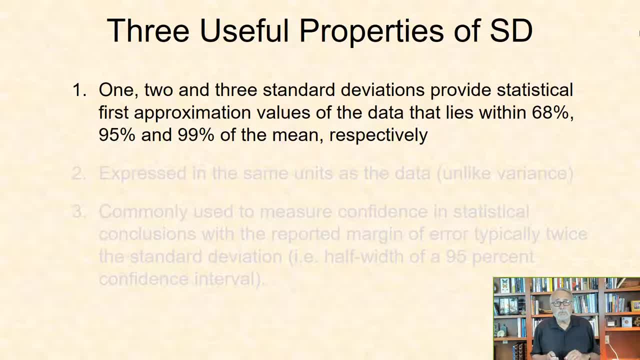 From meta-www margin. we can measure data home with the See or Visit function. It explains the different criteria in the Re distributive frontier. provides estimates of the values of data that lie within different percentages of the mean, Specifically 1,, 2, and 3 standard deviations. provide statistical first approximation values. 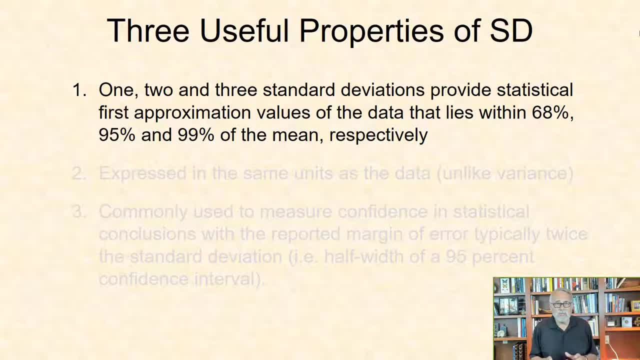 of the data that lies within 68%, 95% and 99% of the mean respectively. Second, standard deviations are expressed in the same units as the data, unlike the variants. For example, 1,000 eggs plus or minus 200 eggs. standard deviation. 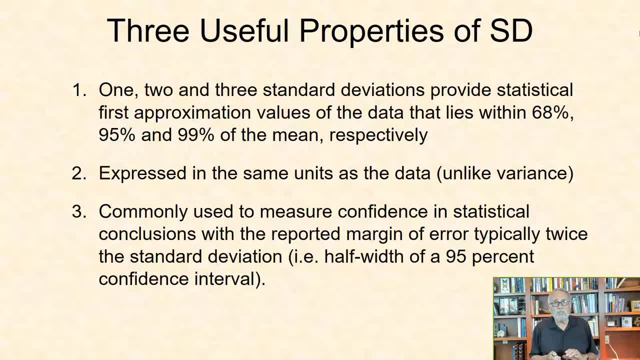 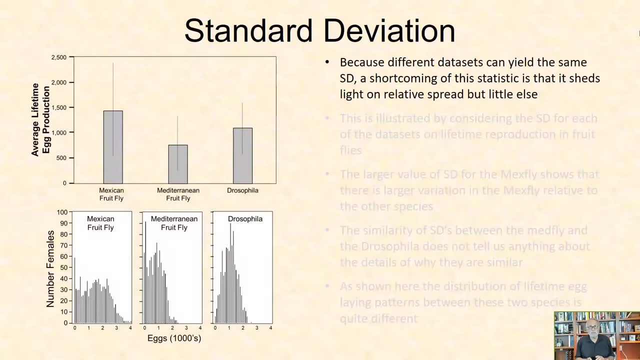 Third, the standard deviation is commonly used to measure confidence in statistical conclusions, with the reported margin of error typically twice the standard deviation, ie half-width of the 95% confidence interval, Because different datasets can yield the same standard deviation. a shortcoming of this statistic is that it sheds light on relative spread. 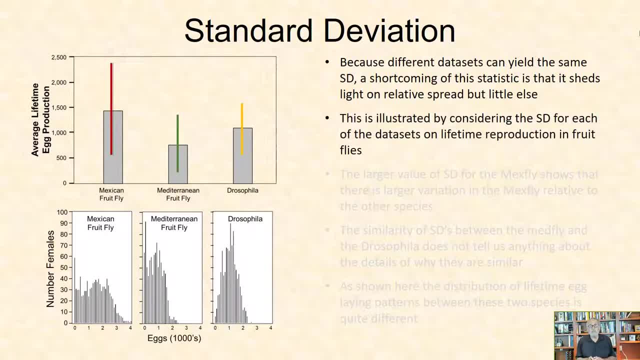 but little estimate. This is illustrated by considering the standard deviation for each of the datasets on lifetime reproduction in fruit flies, Although the larger value of standard deviation for the MEX fly shows that there is larger variation in the MEX fly relative to the other species' reproduction. 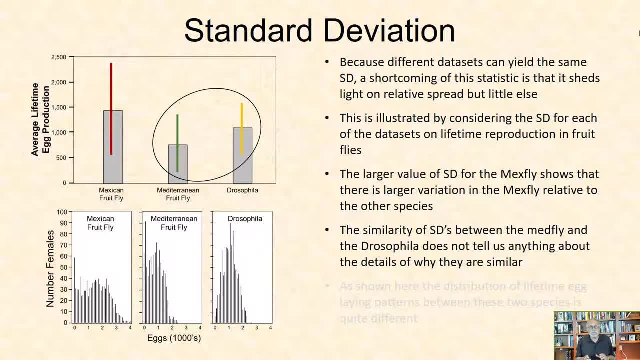 the similarity of standard deviations between the MED fly and the Drosophila does not tell us anything about the details of why they are similar. In fact, as shown here, the distribution of lifetime egg-laying patterns between these two species is quite different. 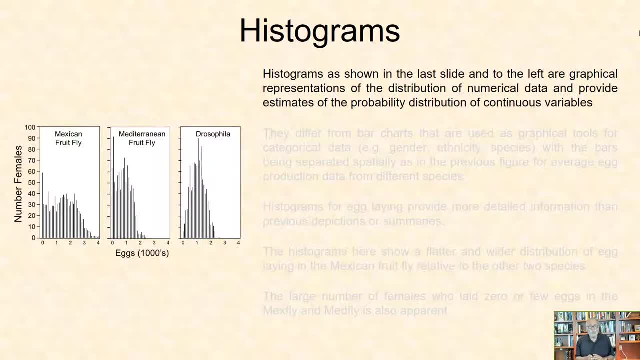 Histograms, as shown in the last slide and to the left, are graphical representations of the distribution of numerical data and provide estimates of the probability distribution of continuous variables such as birth and death distributions. They differ from bar charts that are used as graphical tools. 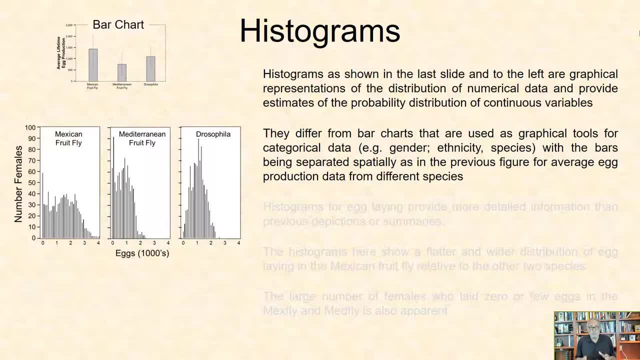 for categorical data like gender, ethnicity, species, With the bars being separated spatially, as in the previous figure for the average egg production data from different species. Histograms for egg-laying provide more detailed information than previous depictions or summaries. For example, the histograms show a flatter and wider distribution. 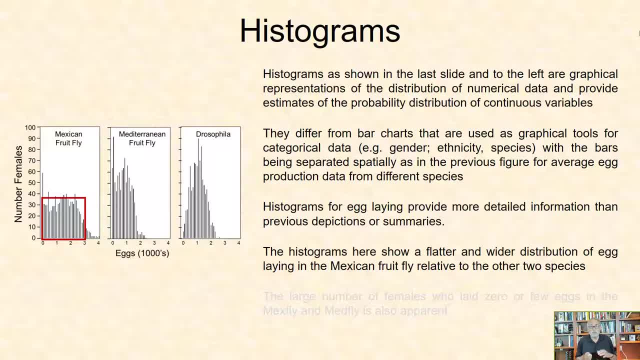 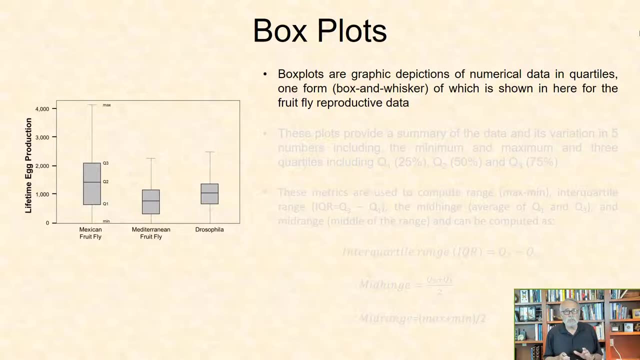 of egg-laying in the Mexican fruit fly relative to the other two species. The large number of females who laid zero or few eggs in the MEX fly and the MED fly is readily apparent. Box plots are graphical depictions of numerical data in quartiles. 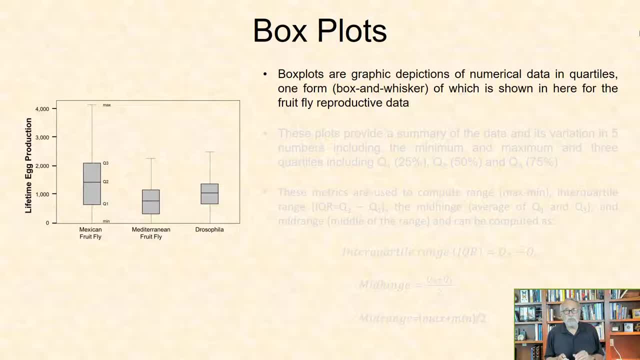 one form being the box and whisker of which is shown here for the fruit fly reproductive data. These plots provide a summary of the data and its variation in five numbers, including the minimum and the maximum, and three quartiles, including Q1, 25%, Q2, 50% and Q3, 75%.